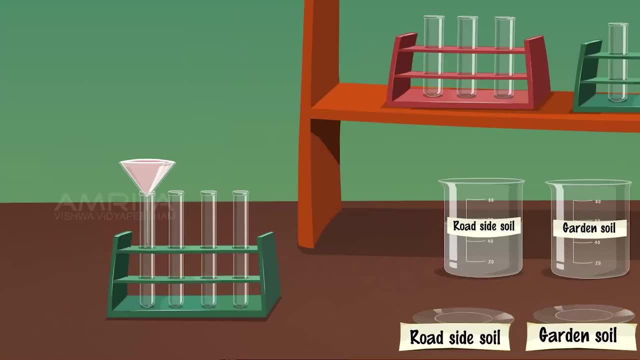 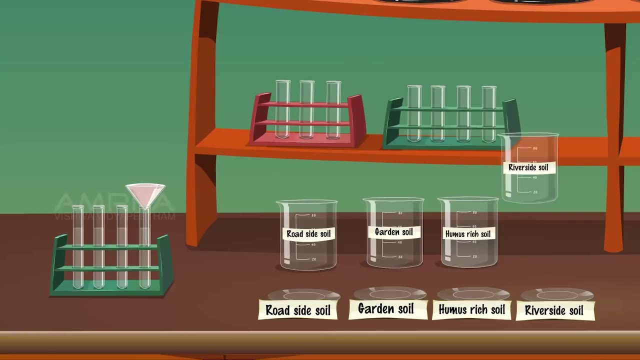 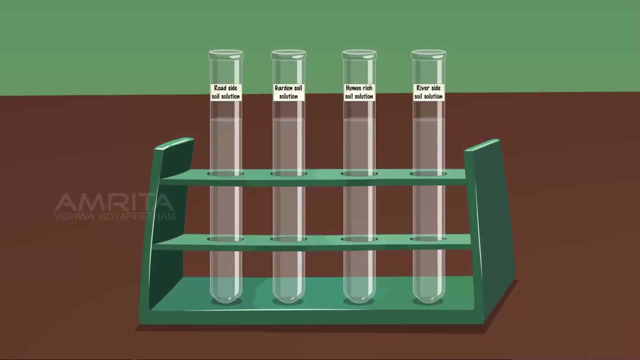 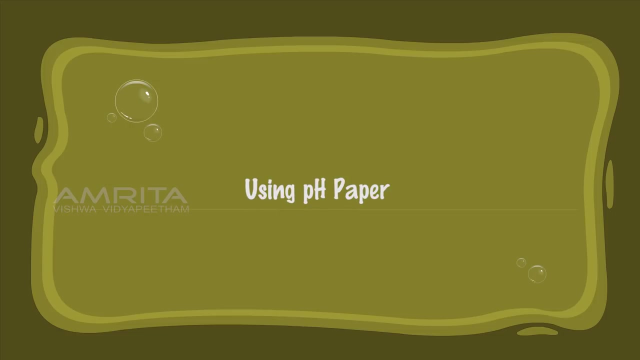 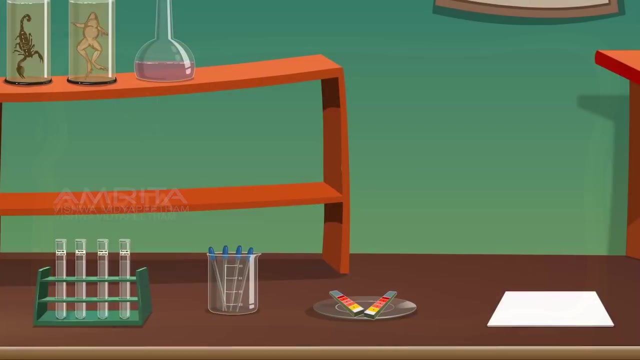 Now take roadside soil solution and filter the solution through the filter paper and collect the filtrates in a test tube. Repeat the same procedure for other samples with fresh filter papers. The soil solution is now ready for testing pH Using pH paper. Materials required Soil solutions. 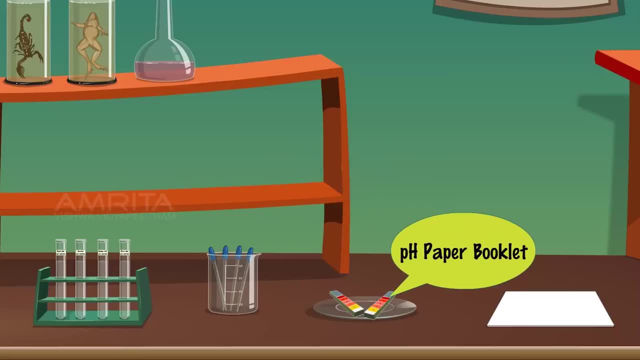 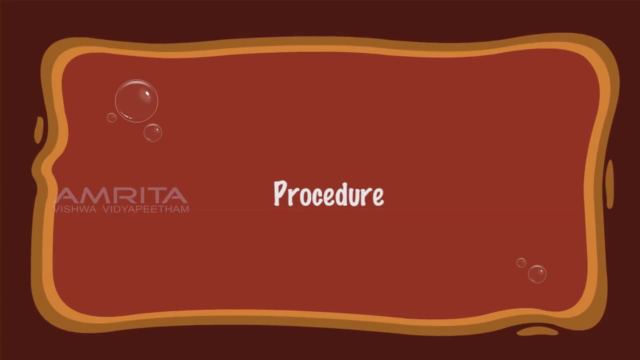 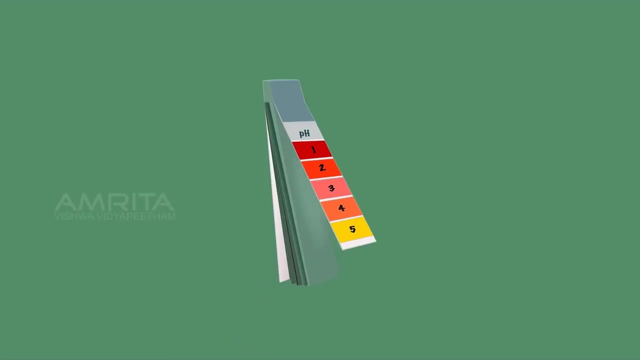 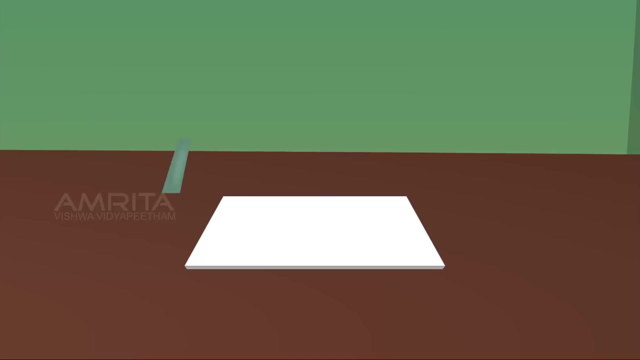 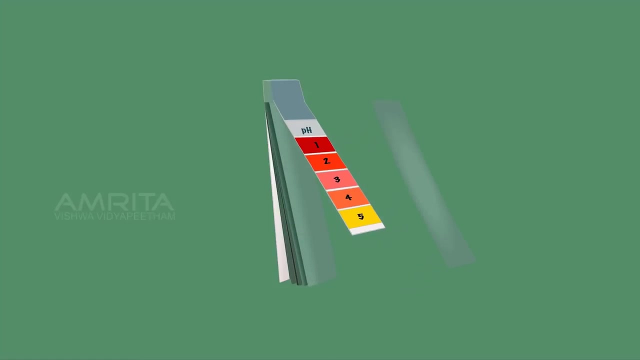 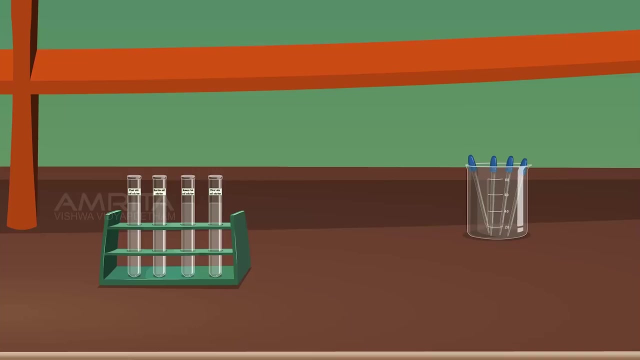 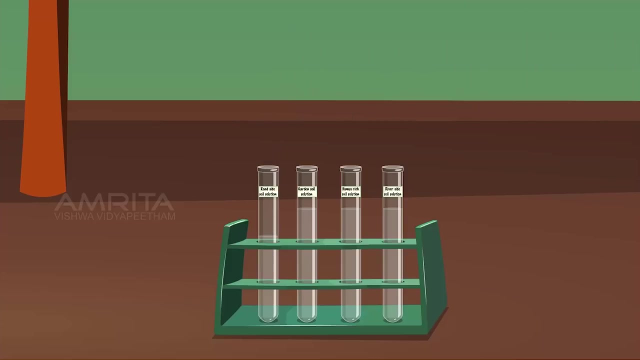 Droppers, pH paper booklet and a tile. Procedure. Take a pH paper booklet, Tear pH paper strips from the booklet and place 4 strips on the tile Using a dropper. take some roadside soil solution from the table test tube. Put one to two drops of solution on the first. 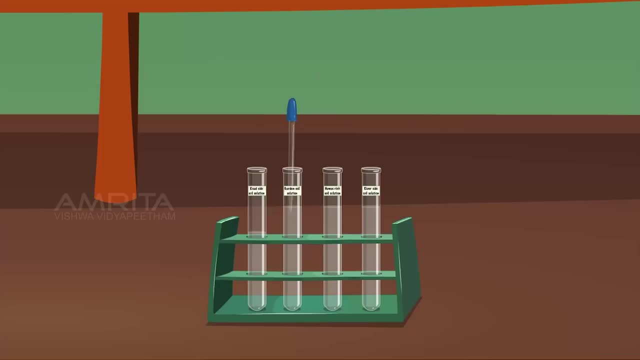 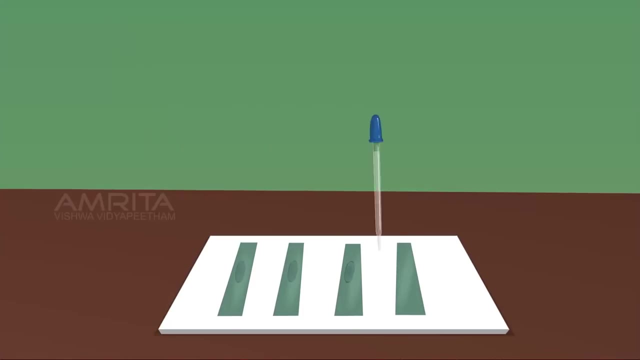 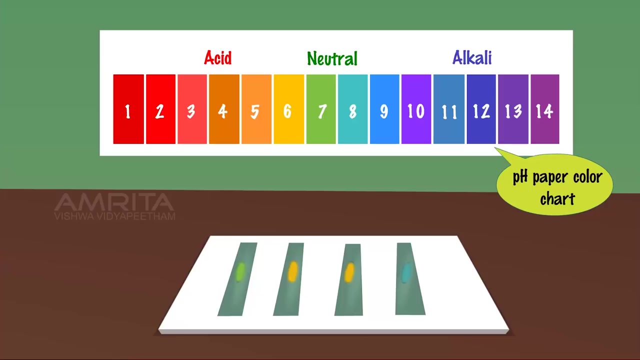 pH strip on the tile Using fresh droppers. do the same procedure for garden soil, humus, rich and riverside soil. Wait for some time for the pH paper strip to dry, Note the colour and compare with the colour chart given on the broad range indicator paper and get a rough estimate of pH of the sample. 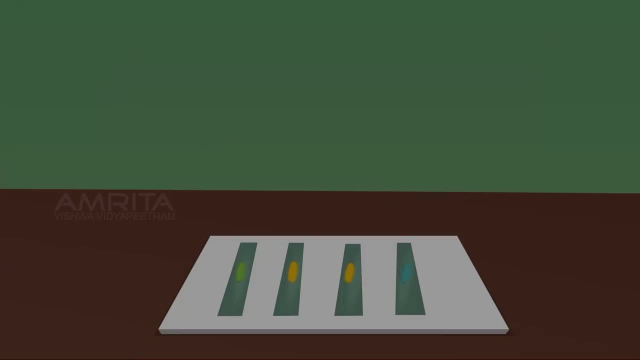 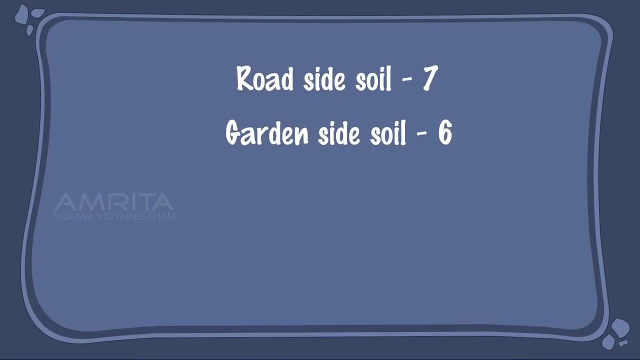 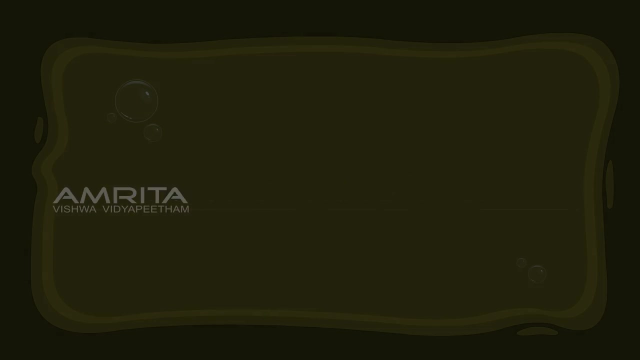 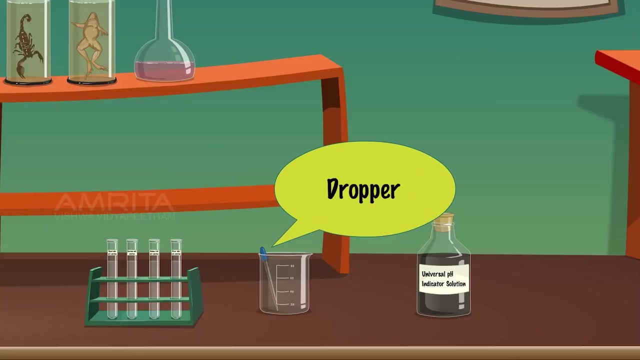 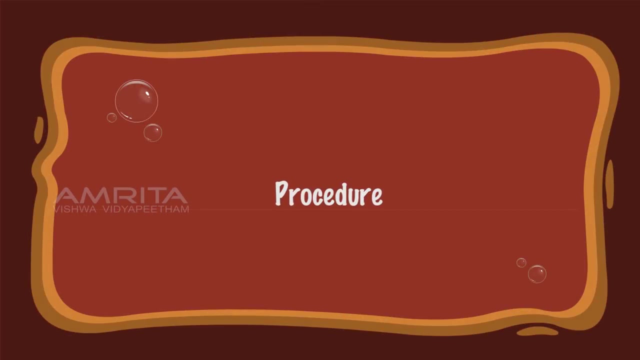 solutions. We can observe that the roadside soil has pH 7, garden soil and humus rich soil have pH 6. And riverside soil has pH 8.. Using Universal Indicator Solution. Materials: Required Soil Solutions, Dropper And Universal pH Indicator Solution Procedure. 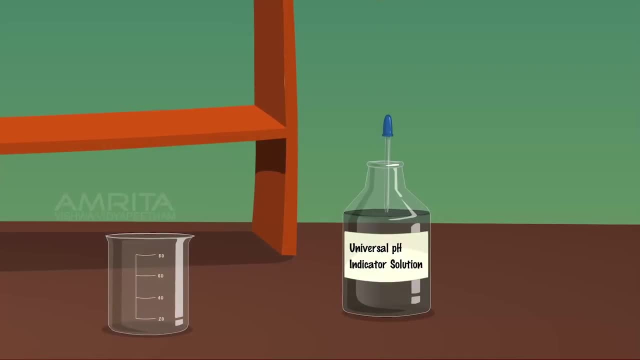 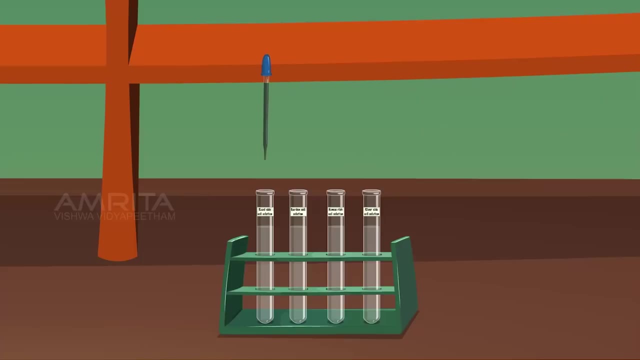 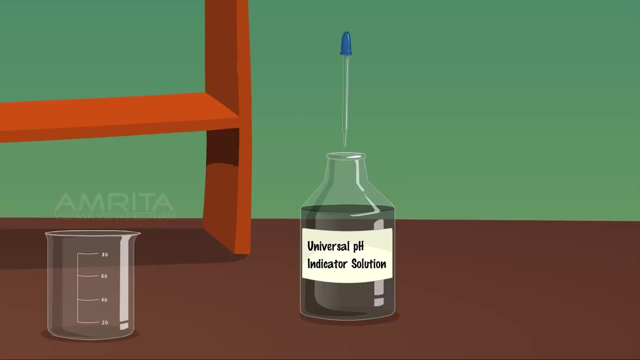 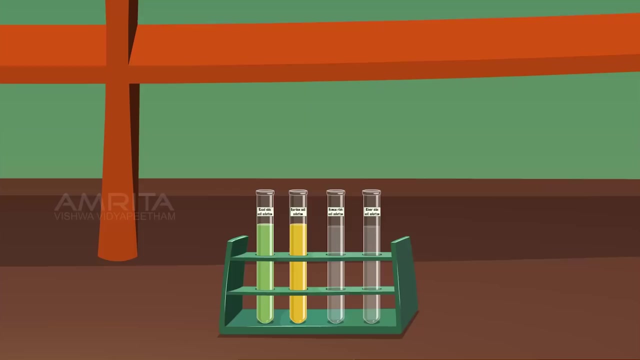 Using a dropper, take some universal pH indicator solution. Using a dropper, take some universal pH indicator solution. Using a dropper, take some universal pH indicator solution. If possible, you may also take the universal indicator solution. Put 5 drops of indicator solution into the test tube that contain water samples from. 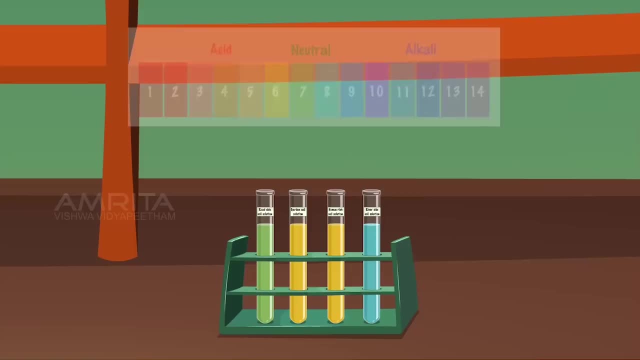 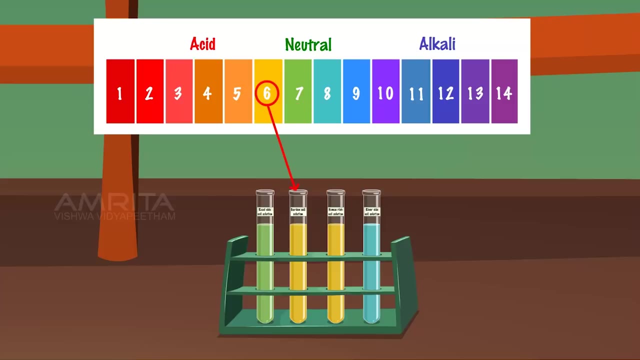 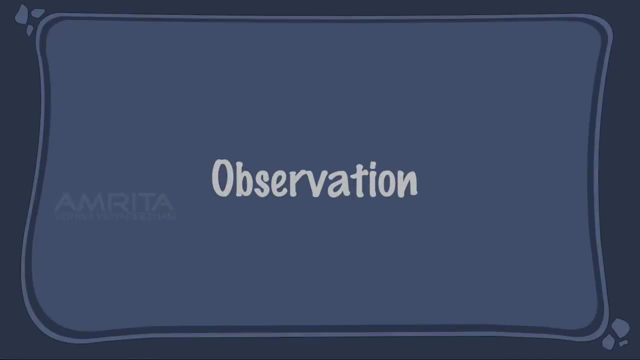 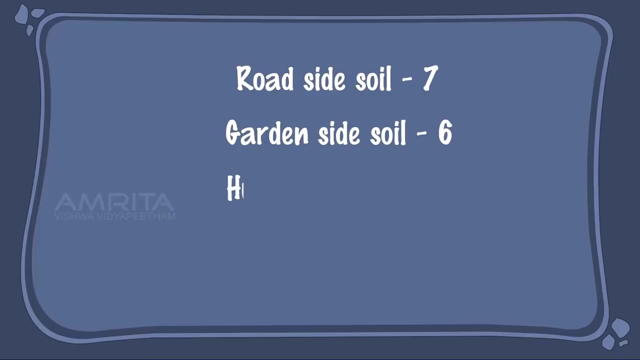 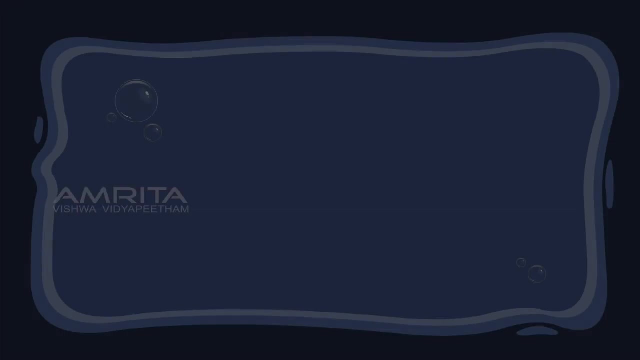 roadside soil, garden soil, humus rich plant soil and riverside soil. In this case you can see œ in the green line Observation. We can observe that the roadside soil has pH 7, garden soil and humus rich soil have pH 6 and riverside soil has pH 8.. 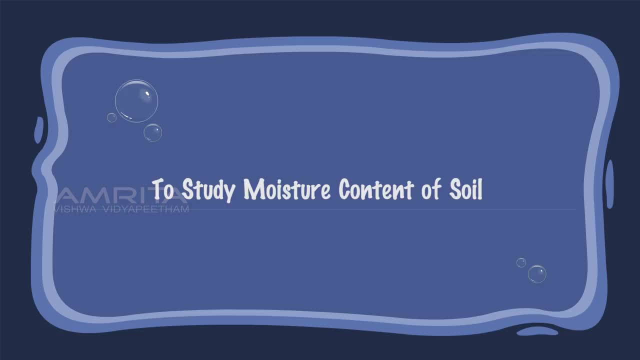 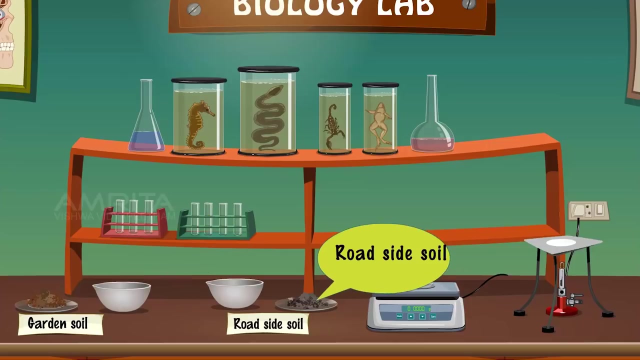 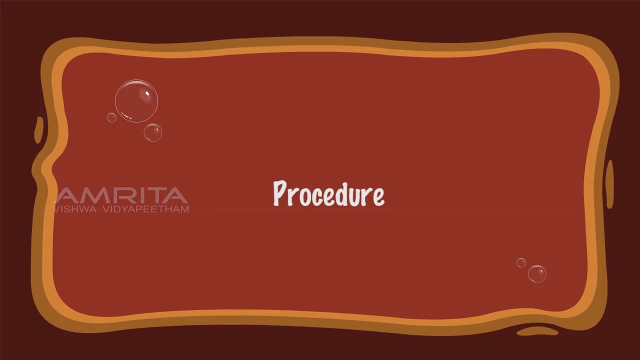 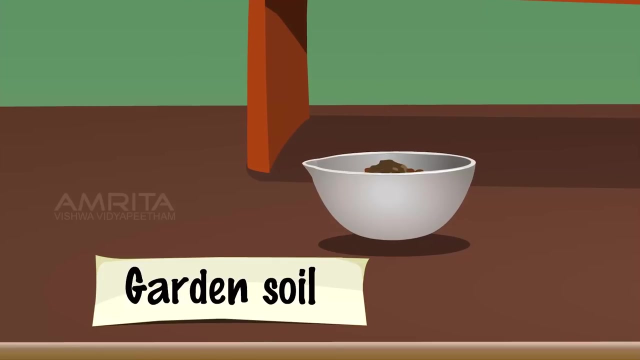 The Static Moisture Content of Soil. Materials Required: Garden Soil Crucibles, Roadside Soil Weighing, Balance Burner and Wire Gauze. 1. Static Moisture Content of Soil Procedure: Take watch glass containing garden soil and put it into a crucible. 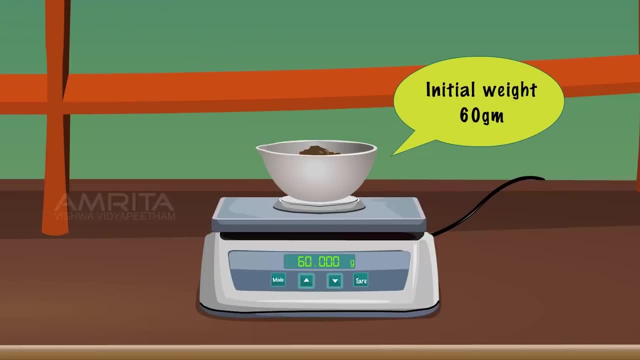 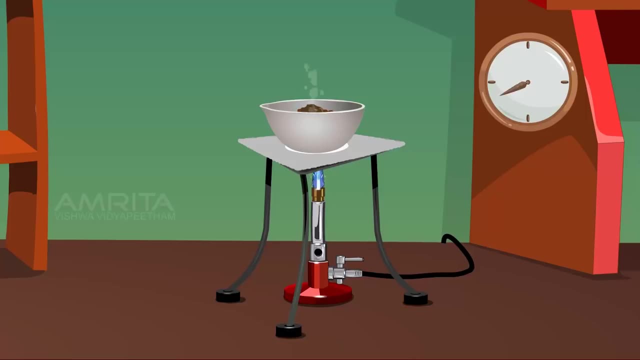 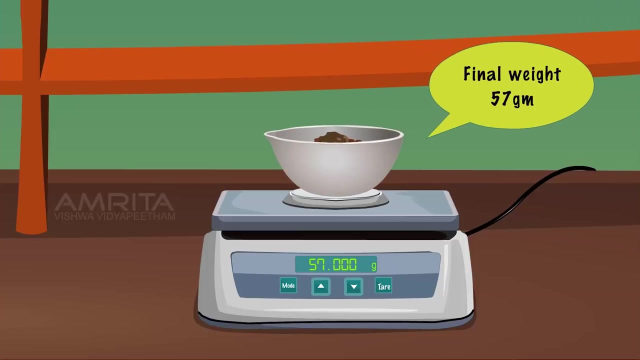 Weigh the crucible with soil sample on a weighing balance. Take crucible and place it over the Bunsen burner. Heat the soil for some time till the soil becomes dry. Weigh the crucible again to record the weight of dry soil. 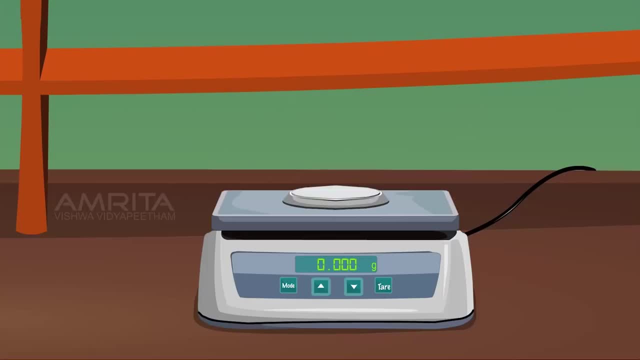 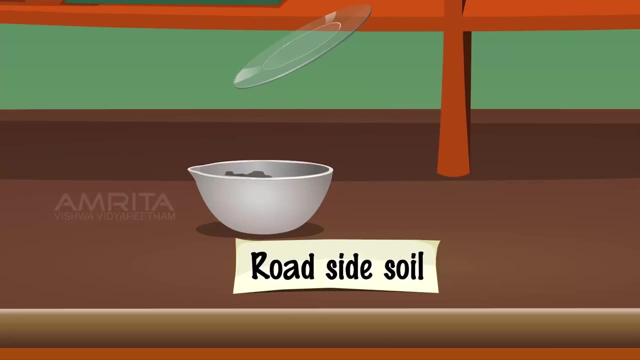 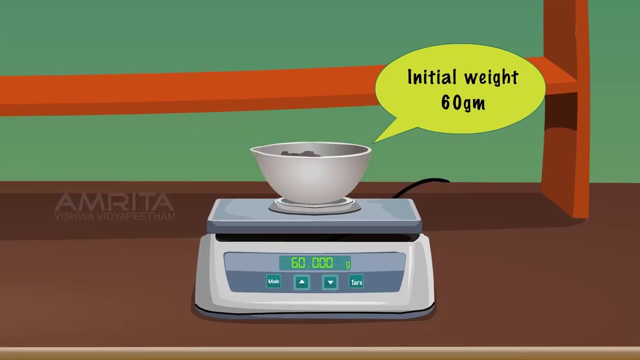 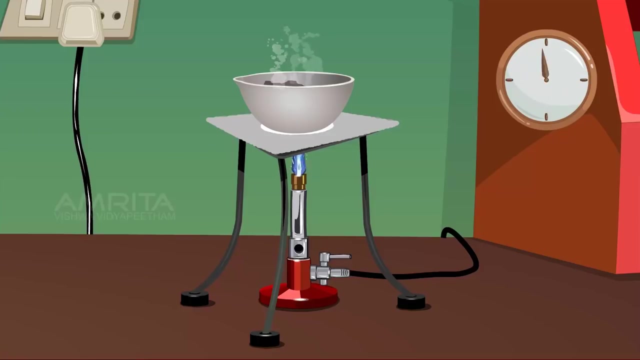 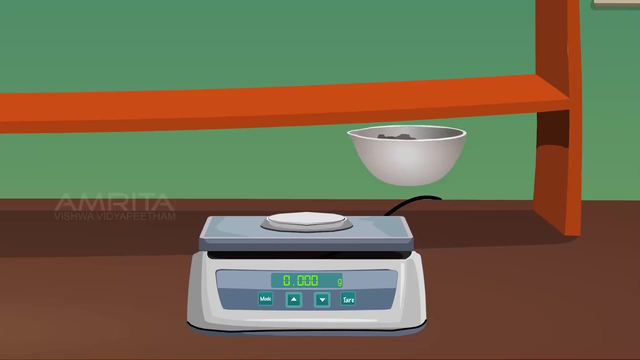 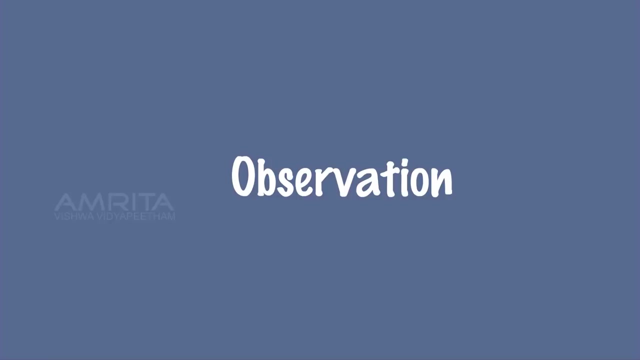 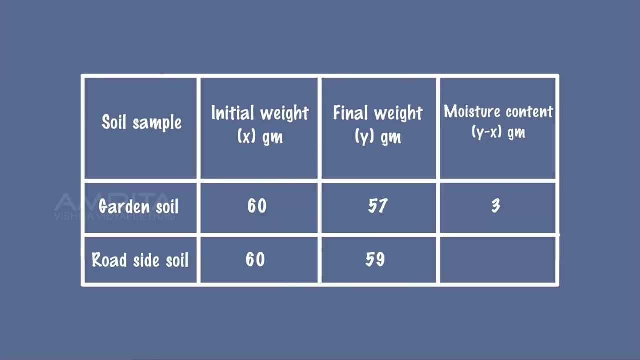 2. Spats. 6. Dosage: Take a transfer 건ược of dry soil. 3. Weigh the crucible again to record the weight of dry soil. Observation: Record the initial and final weights of each sample and the difference between initial. 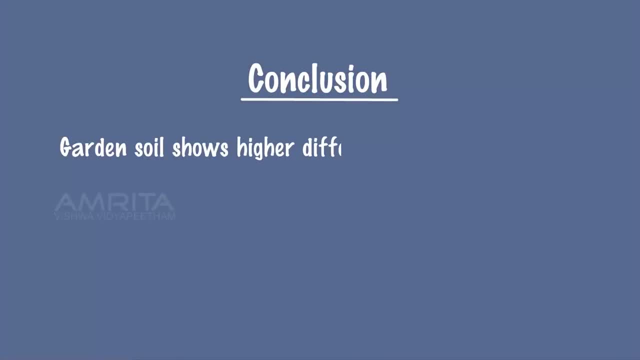 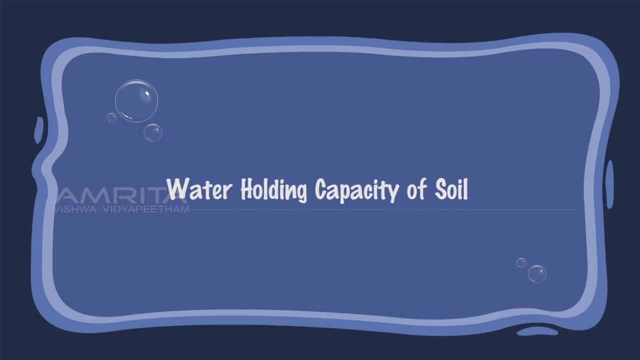 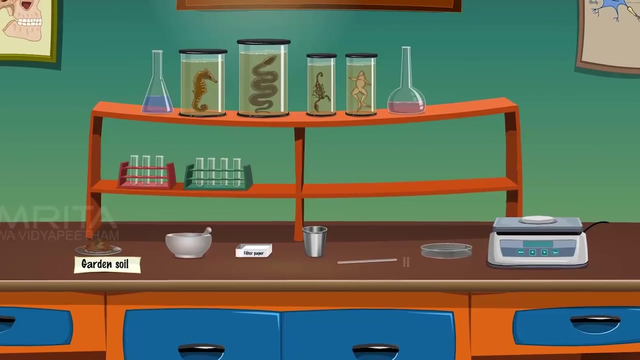 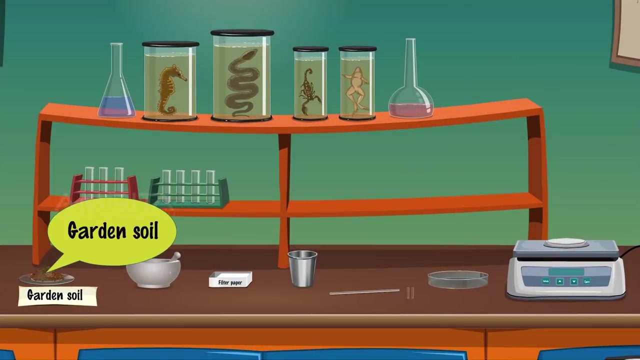 and final weights in the form of a table. Conclusion: Garden soil shows higher difference between initial and final weight, indicating higher moisture content in the garden soil than the roadside soil. Water Holding Capacity of Soil Materials: Required Soil Sample from Garden Mortar and Pestle Filter Paper. 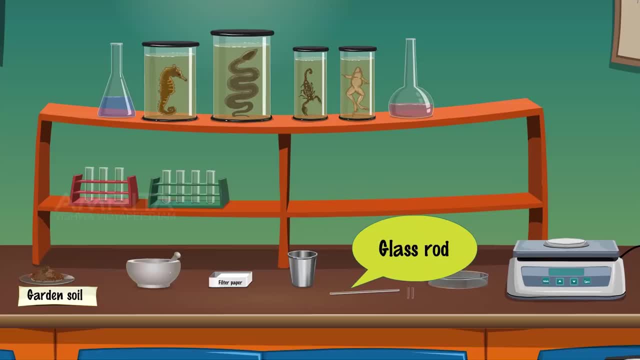 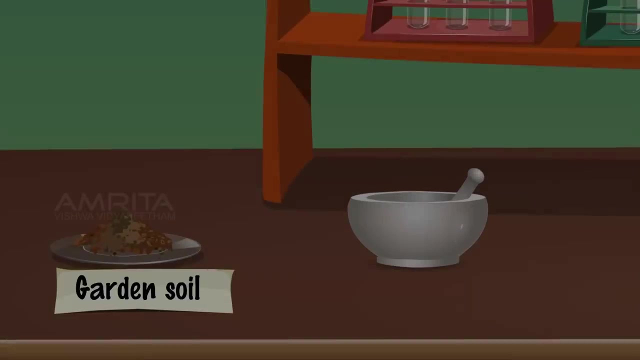 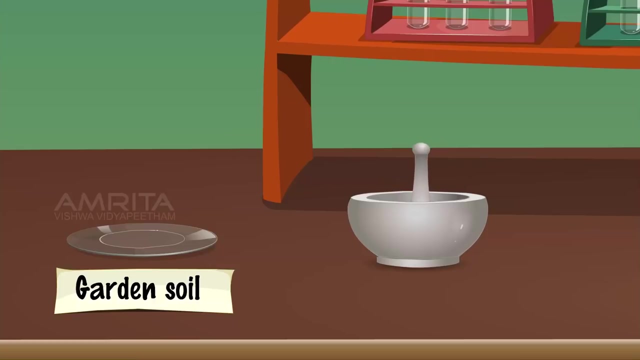 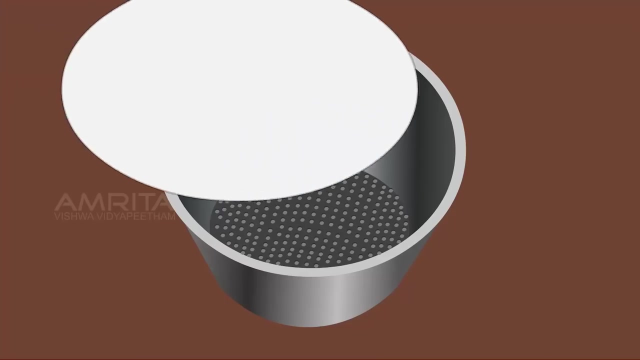 Tin Boxes with Perforator Rated Bottoms. Glass Rod, Small Glass Rods, Petri Dish Weighing Balance Procedure. Take a watch glass containing garden soil and put it into a mortar. Using a pestle, grind the sample into fine powder. Take a filter paper and place it in the bottom of the pot. 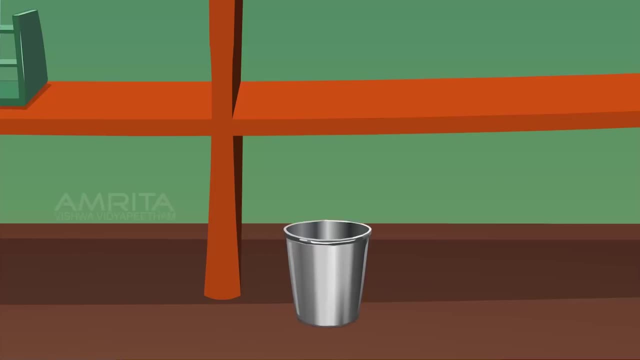 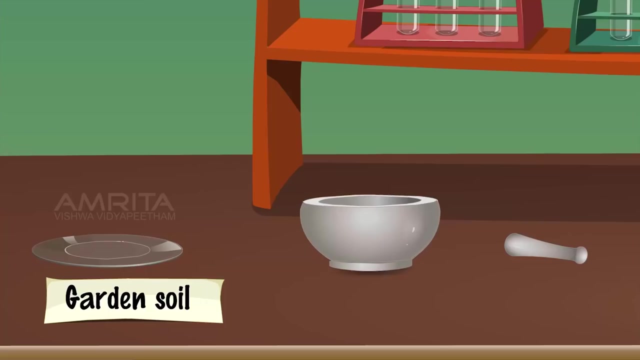 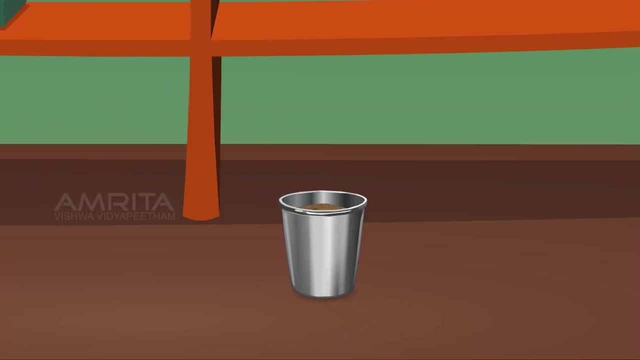 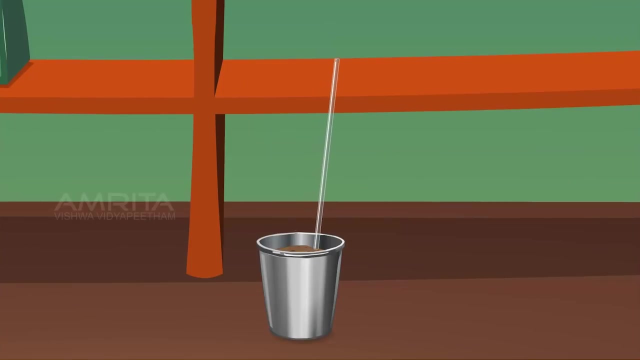 Weigh the tin box along with the filter paper and note its weight. Transfer the fine powdered soil sample into the tin box. Take a glass rod and tap the box gently several times so that soil is compactly filled and forms a uniform layer at the top. 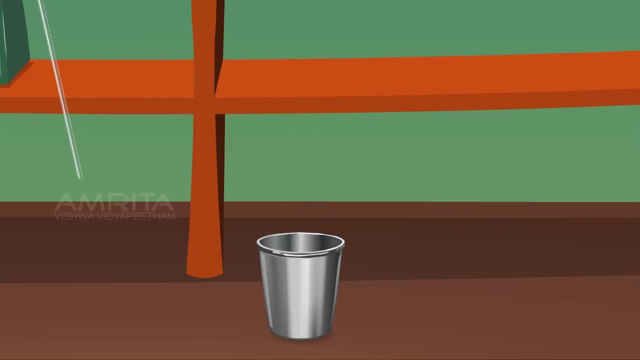 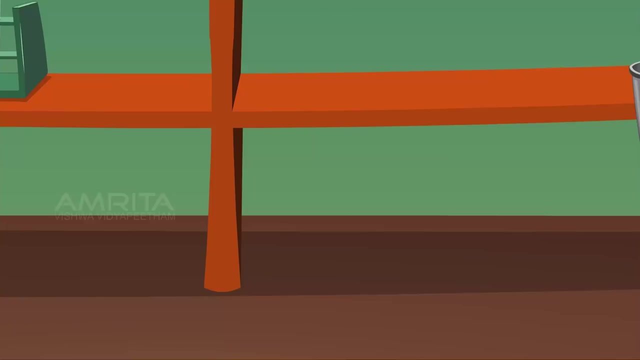 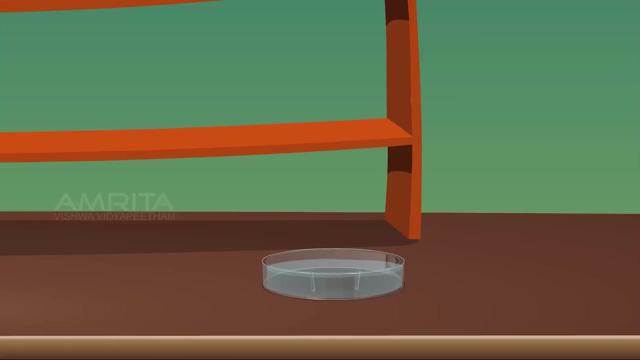 Weigh the tin box along with the filter paper and note its weight. Transfer the fine powdered soil sample into the tin box. Weigh the tin box along with soil sample and note its weight. Take a petri dish filled with water. Take two small glass rods and place them parallel to and at a small distance from each other. 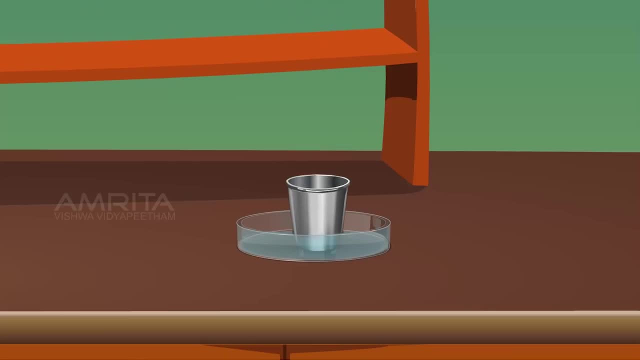 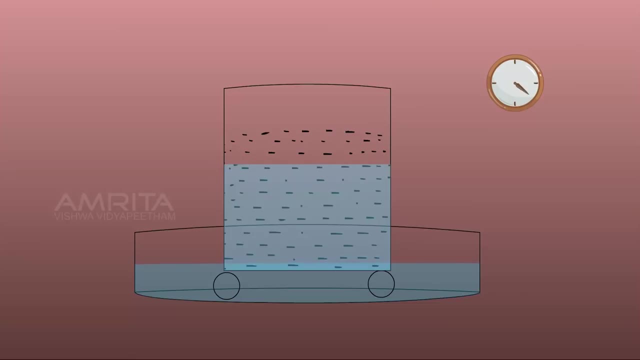 Place the soil-filled tin on the two glass rods in such a manner that its bottom is in contact with water. Leave the set up undisturbed till water appears on the upper surface. Place the tin box on the bottom of the pot. Wait a few seconds. 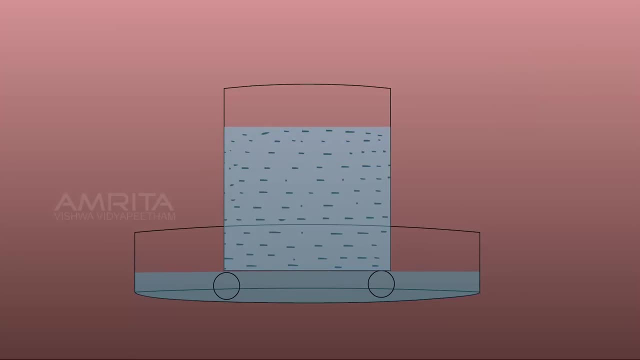 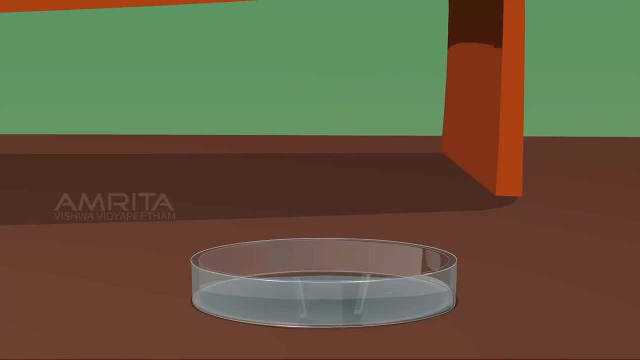 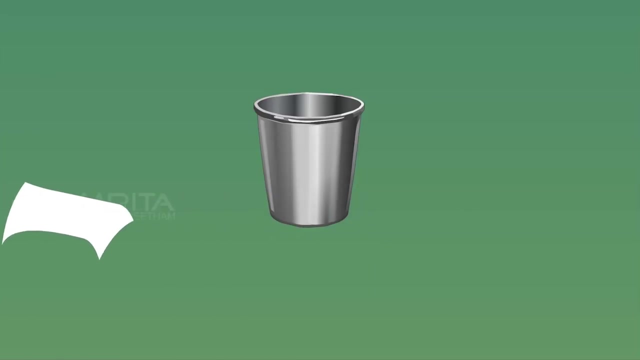 surface of the soil. Wait till the entire soil surface is wet. Remove the tin and allow all the gravitational water to flow out from the bottom. When no more water percolates, wipe the bottom to dry it with a filter paper. Weigh them again and note its weight.